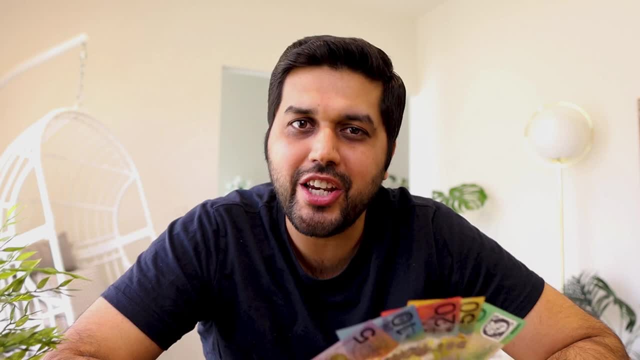 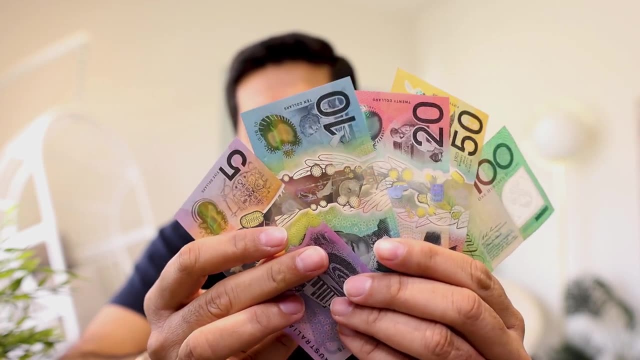 in regards to these lovely bank notes. Now, before we talk about the features, I just want to talk about what these bank notes actually are. I mean, if you look at any of these bank notes- so just as an example, let's look at this $10 note- I mean, what do you guys think I think this bank note? 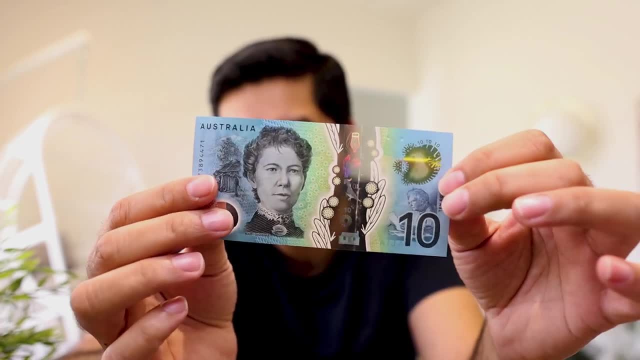 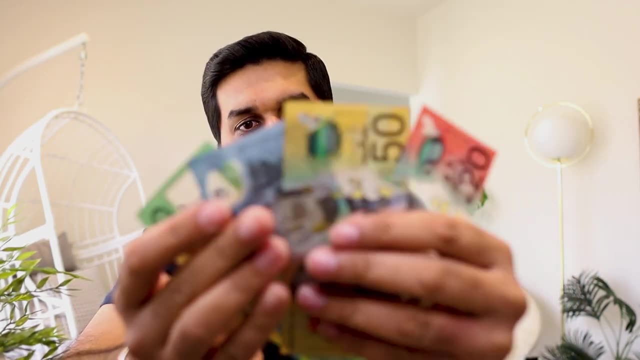 really looks beautiful. I would love to hear your thoughts on that in the comment section below. And we can say the same thing about all other bank notes as well. The way they have designed it and they have printed it, and the colors- they are just all beautiful, Now, apart from just being beautiful. 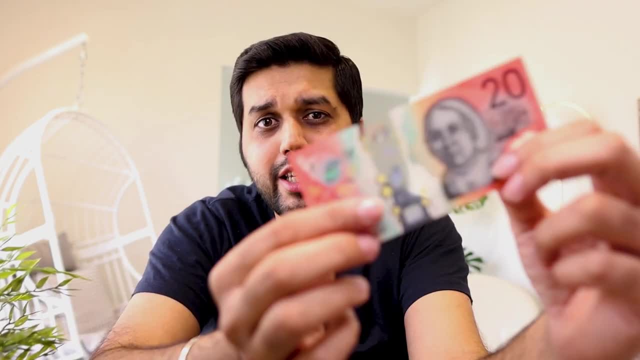 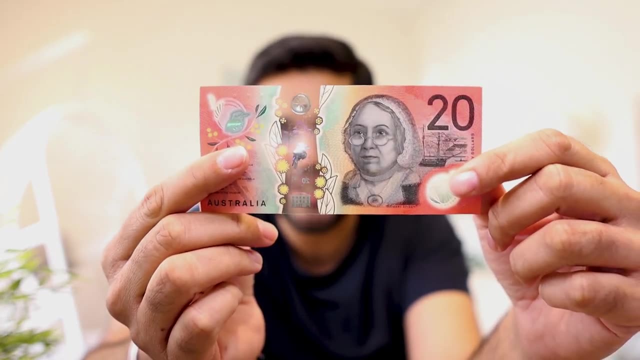 there are many other features that you will see. First thing first, as these bank notes are made from plastic or polymer, they are very, very durable, And I will show you that in the next few minutes with our stress test: how durable they actually are. Now, apart from being durable, 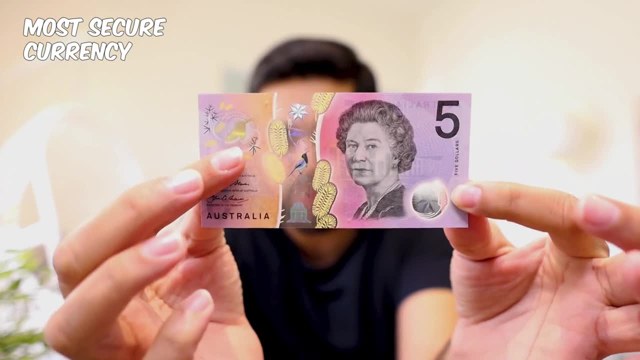 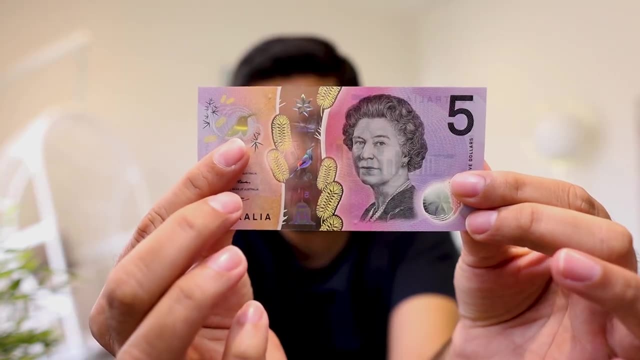 these are some of the most secured currencies in the world as well, And there are very little counterfeit or fake notes out there for this currency, And the biggest reason for that is the way it is being printed- which we'll talk about it in a few minutes- And these notes tend 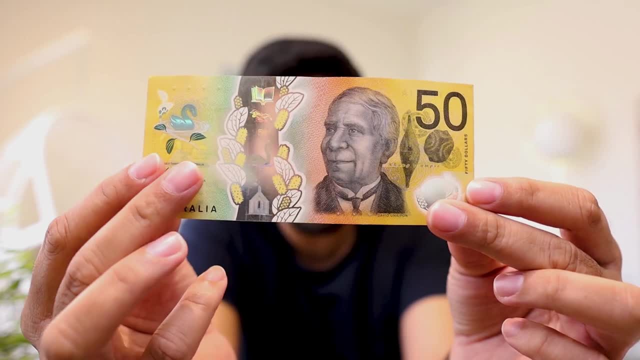 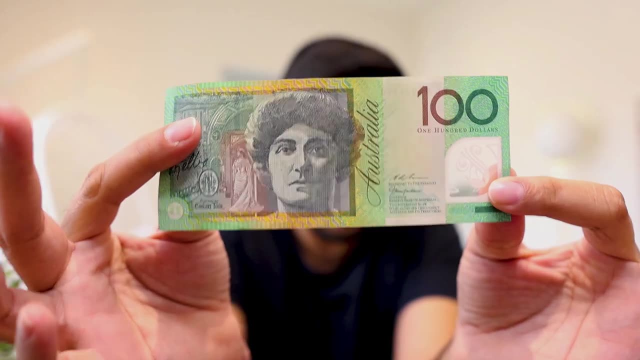 to be paper bank notes. An average lifespan of this one currency note is around seven years, which is quite a lot comparing to paper and cotton bank notes that we see around the world, And after the usage is finished, they can be recycled again, So they are considered to be. 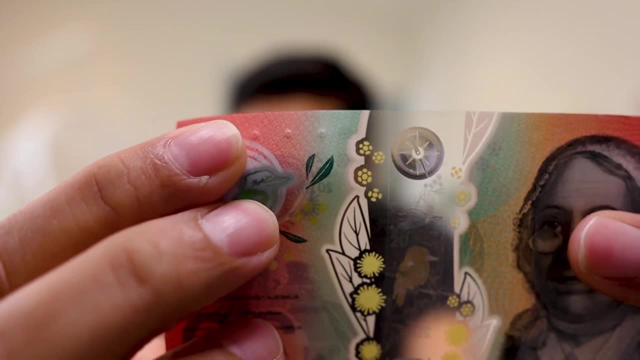 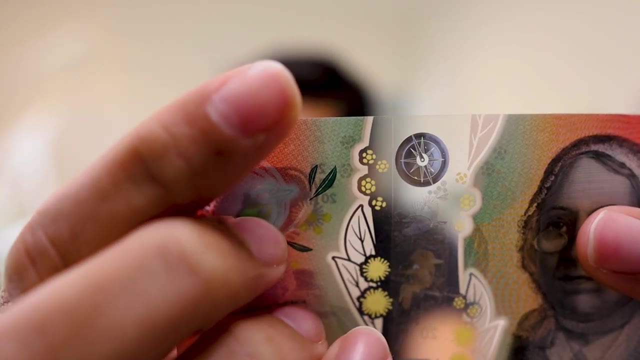 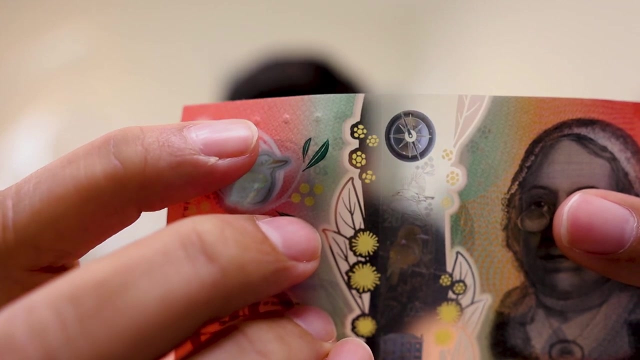 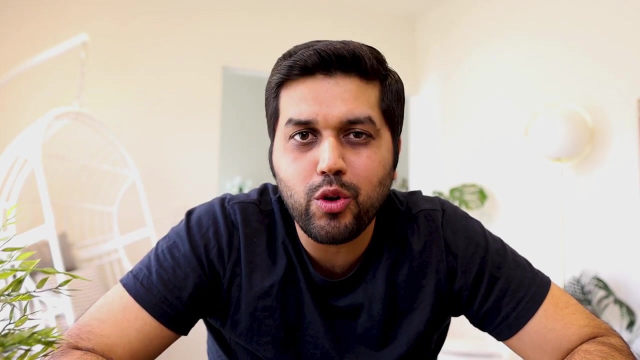 one of the most environment friendly notes in the world as well, And to make it accessible for everyone, the government even have these tactile features in these new bank notes as well, especially the one launched after 2015 onwards. Now let's have a quick look at each of these bank notes and see what are some of the features in. 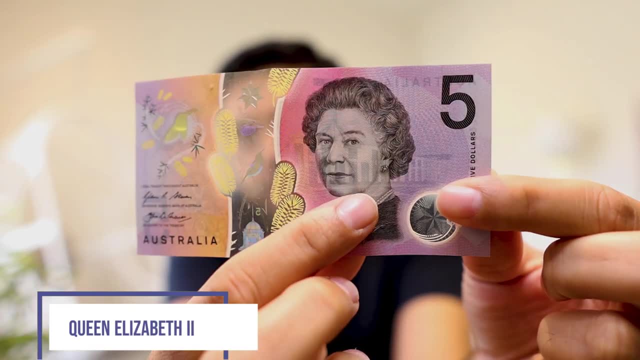 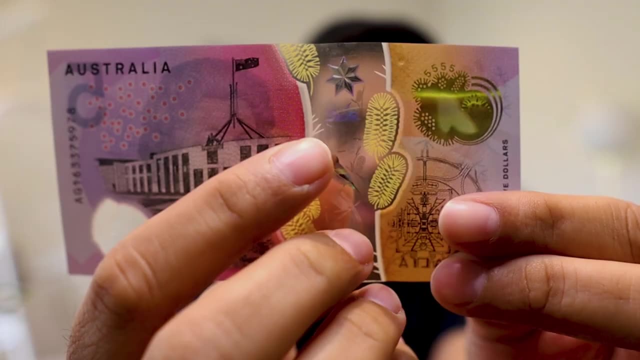 these bank notes. First thing, with the $5 note you will see the photo of Queen Elizabeth II, And on the flip side you will see the Australian Parliament. At the top you will see this Federation Star. Then you see this little bird, also known as Pine Hill, right in the middle. And 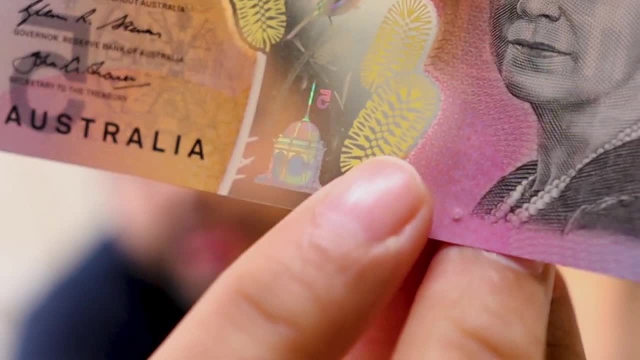 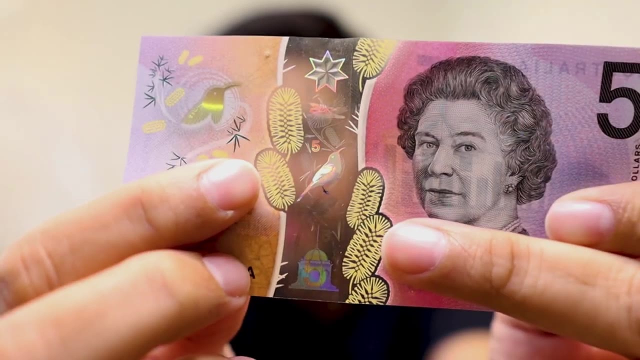 right at the bottom you see Federation Pavilion, And with this holographic image, you can even see $5 being printed right in the middle of this hair as well, And these yellow bottles as well, which are part of Australian's nature. Now let's look at a $10 note On one side of this note. 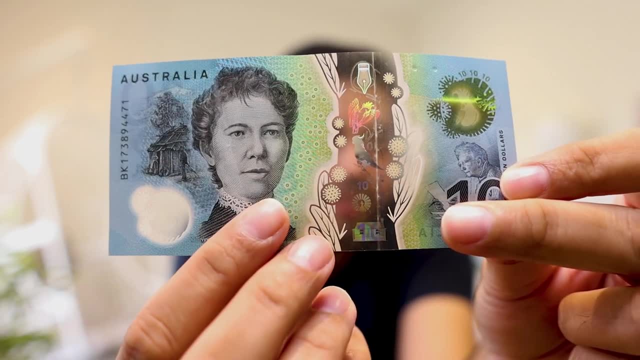 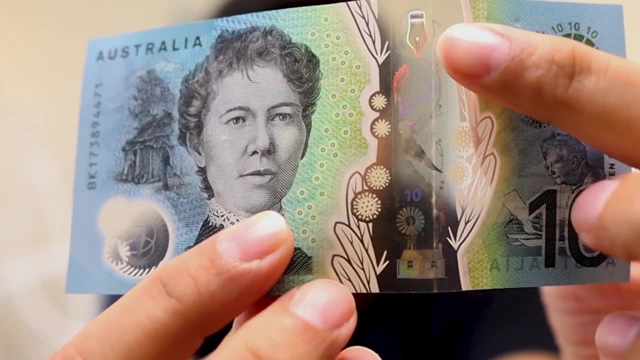 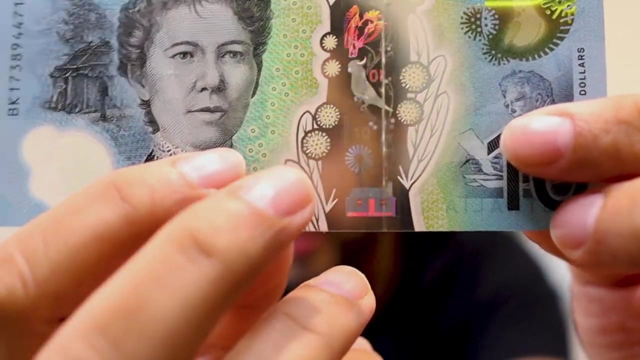 we have Mary Gilmore. She was a famous Australian writer, a journalist and women's right activist. We have her photo over here as well And the holograms we see right at the top, a pen nib. at the bottom Again, you can see $10 featuring in the middle here as well, And there is a text. 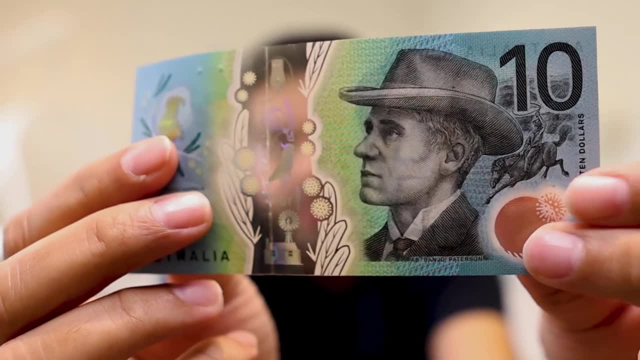 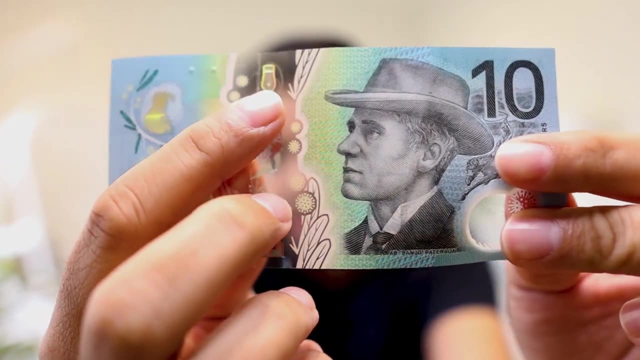 as running in there in the middle of this window as well. On the other side of the bank note we have Banjo Paterson. He was a famous Australian poet and an author And that's why there is a nib here at the top to give respect to both of these poets, And there is a nib on this side of the note. 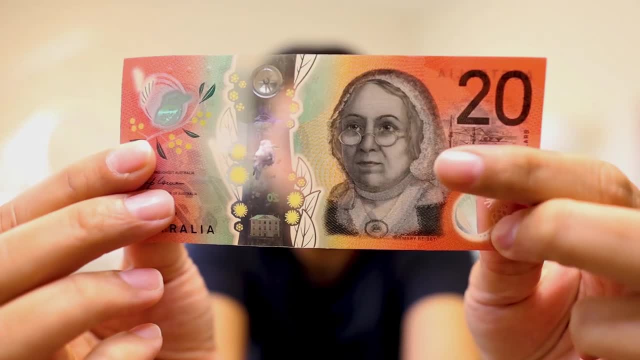 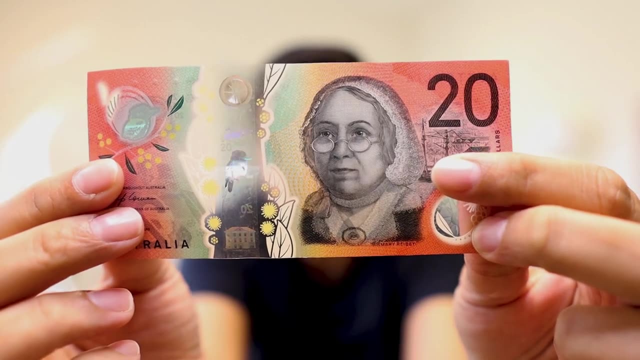 as well. Let's move to the $20 bill. So on this side of $20 bill note we have Mary Ribby. She was a famous woman and a trader and she was also a philanthropist. And if we turn around the note, 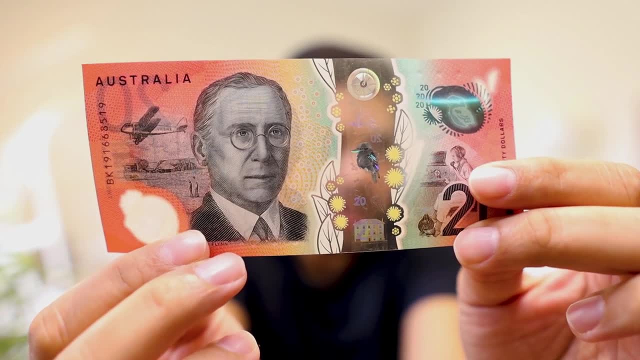 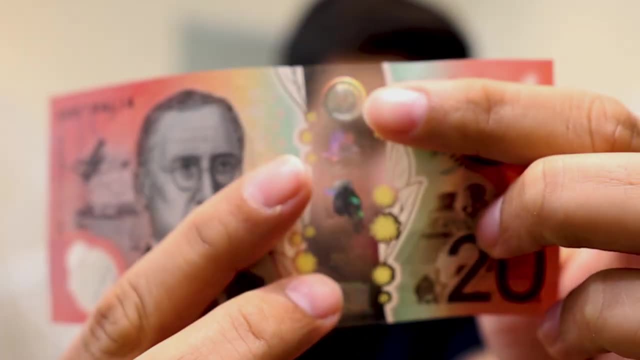 we will see John Flynn, a person who founded the Royal Flying Doctor Service of Australia. Now, if you look around in the holographic side of the things, we have 3D compass at the top, then we have a kookaburra in the middle and then we have at the bottom. 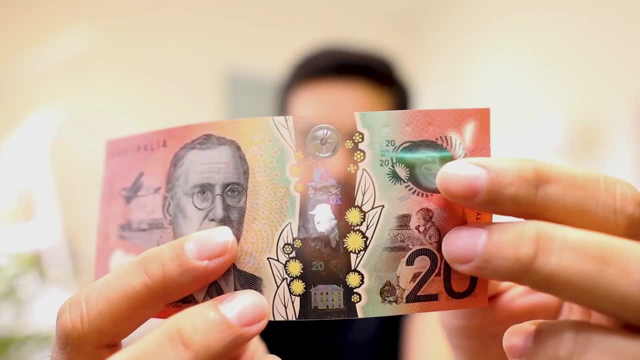 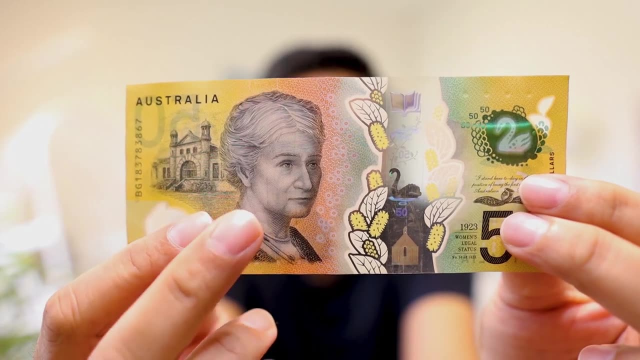 Ribby's Macquarie Place House. Again, there are holographic features and there is a window embedded into this currency note as well. And now let's move to the $50 bill. So on this side of the $50 bill we have Edith Cowan. She was the first woman to be elected to the Australian. 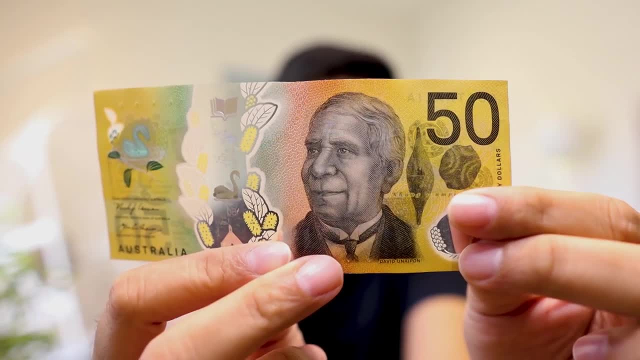 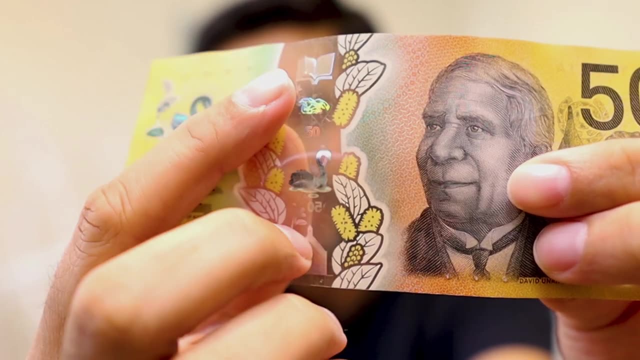 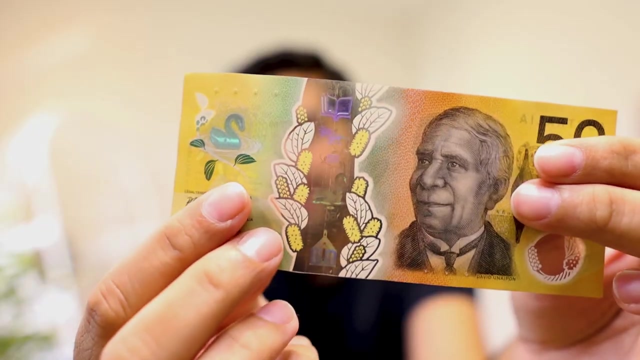 parliament. On this side we have David Winnepon. He was a famous Australian inventor, writer and a preacher, And if you see these holographic images, we have a 3D book here at the top. We have a black swan in the middle here and then we have a church at the bottom, here And again. 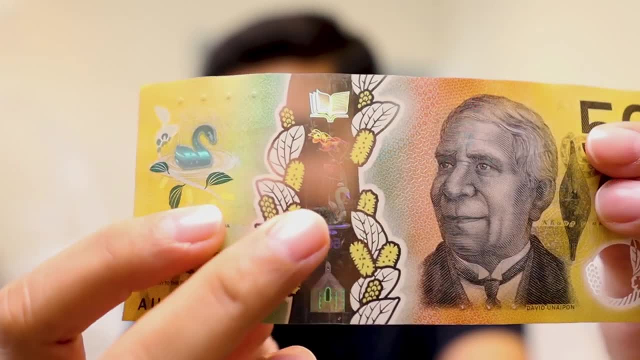 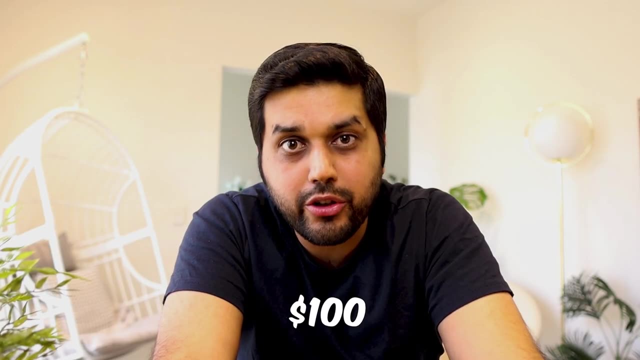 these holographic. if you move them around you can easily see some of these holographic images and numbers and writings in the middle as well. Last one on our list is $100 note. Now I couldn't get a hold of a brand new $100 note because they are in circulation, but sometimes 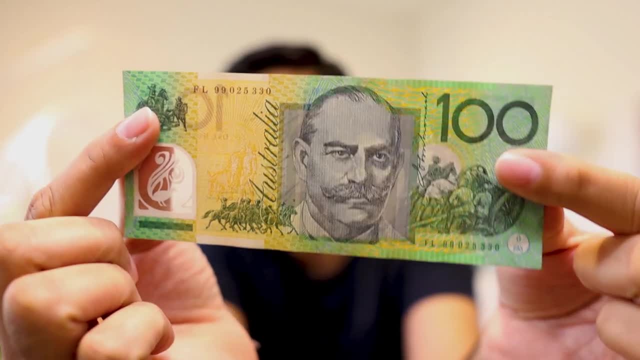 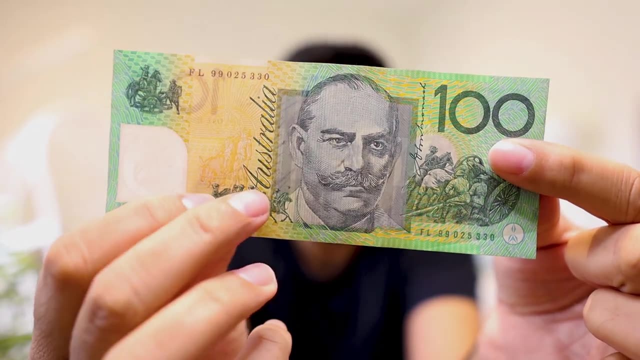 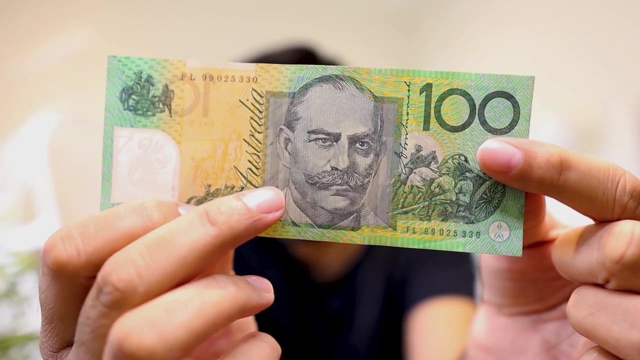 they're hard to find. But here we have the older version of $100 note And that's where you can see the difference between these notes and the newer ones. So on this side of the note we have Sir John Monash. He was a famous Australian military commander who was also involved in Gallipoli. 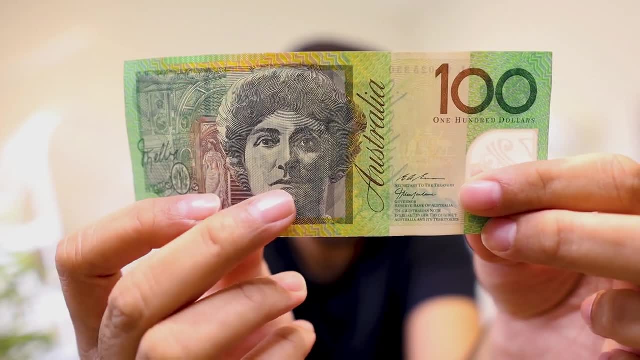 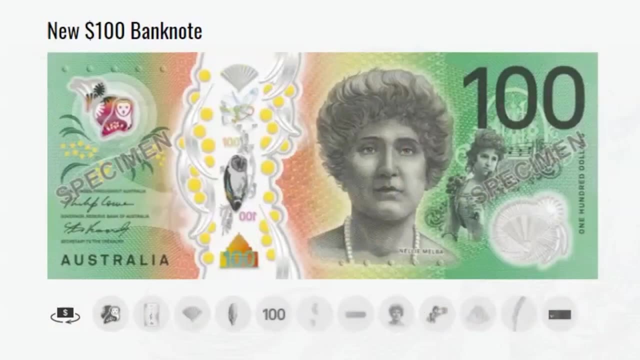 If we turn around this note, we have Nele Melba, an Australian opera singer. She was known for her soprano voice. Here is a quick image of how the newer $100 bill looked like. So in the newer $100 bill you can see 3D fan at the top, Then you have owl in the middle And at the bottom you see. 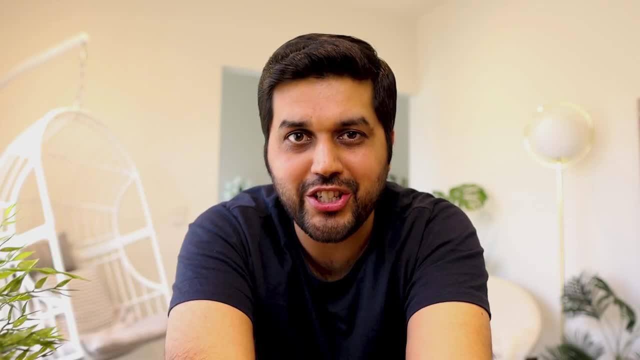 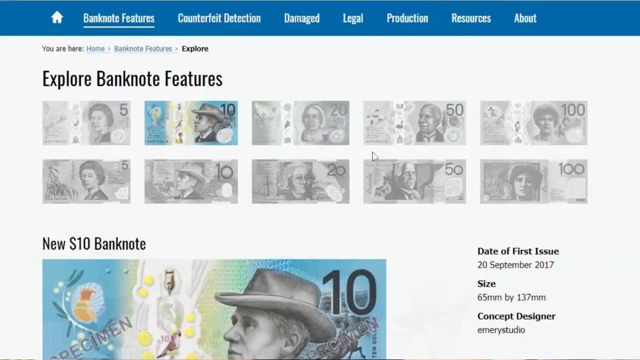 Shrine of Remembrance. Now, obviously, there are a ton of other features in these banknotes which is mind boggling. If you want to know every single one of them, I highly recommend you to check the website, which is Reserve Bank of Australia, And their website includes all the features they have. 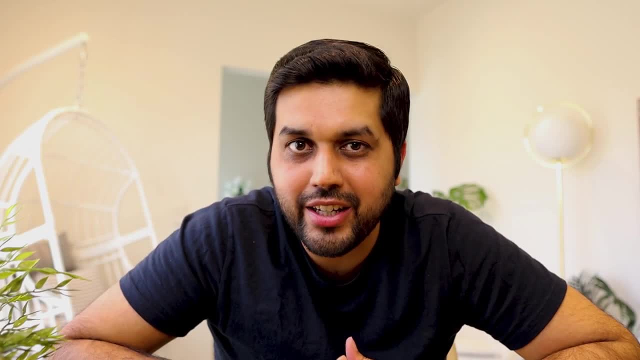 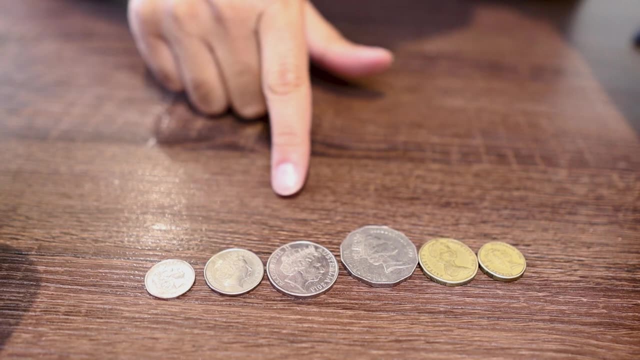 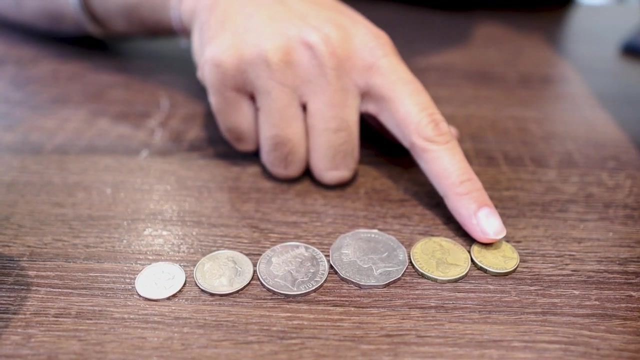 in these Australian notes. And while we are talking about Australian currency, it's not just about the notes. We also have coins as well. These are all the coins we have here in Australia, starting with $0.05,, $0.10,, $0.20,, $0.50,, $1 and $2.. If you see, on the head side of these coins: 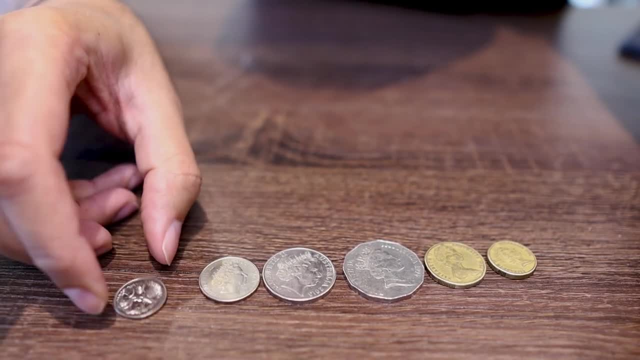 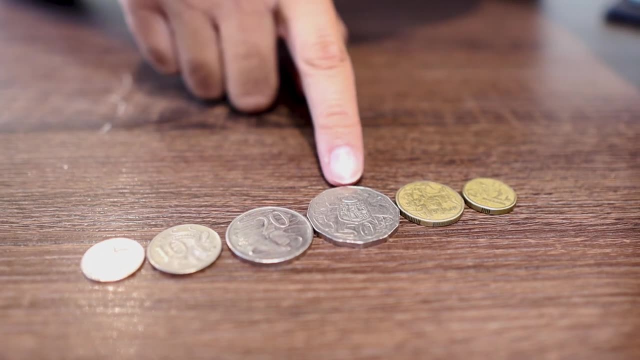 there is Queen Elizabeth II's photos And if you turn them around you'll see Australia's nature, history and flora and fauna. One interesting thing about these coins, especially this $0.50 coin, is that it has 12 sides. So, again, it's very difficult to counterfeit. 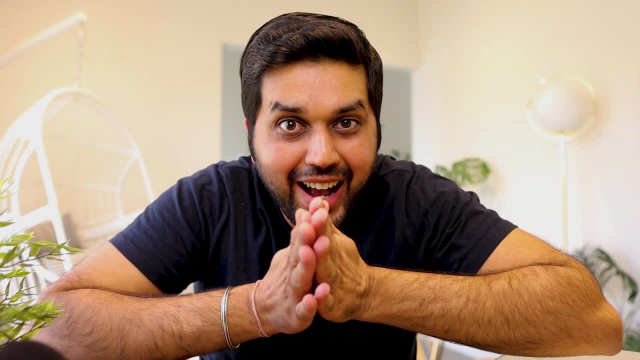 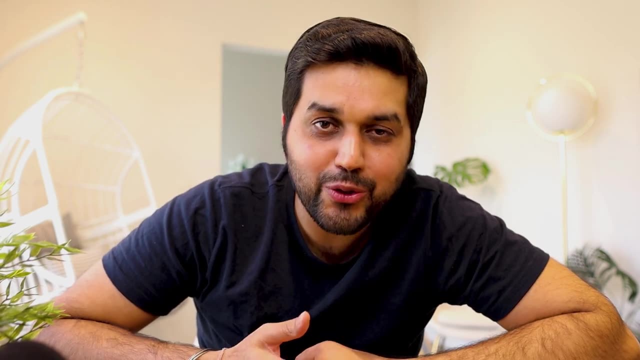 Now, before we move to the final part, which is stress testing- the fun part- I just want to say that these days, many people are not using these banknotes, which, in reality, is a bit sad, because how beautiful these banknotes actually are, I just feel that they should be used more often. 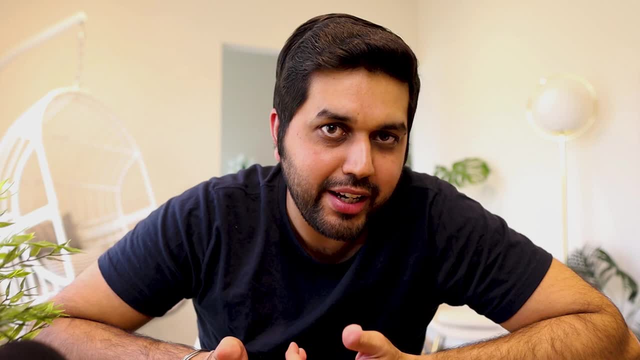 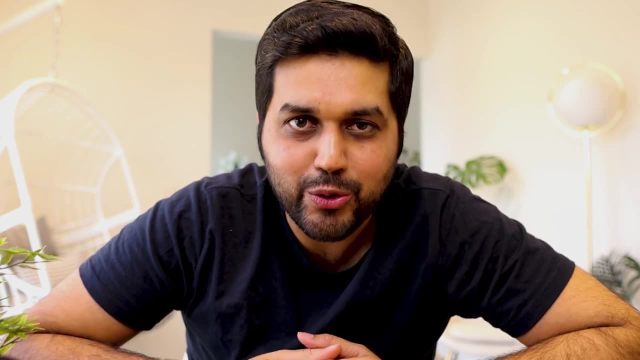 because most of the people these days have started using plastic money. you know cards and Apple Pays and contactless payment methods, which means less and less banknotes are in use, Although if you are coming to Australia, you can easily find ADMs and if you want,